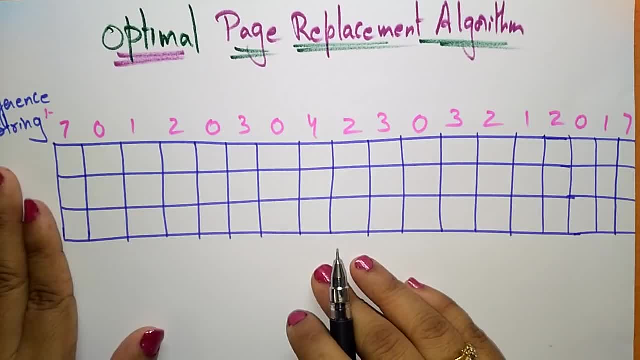 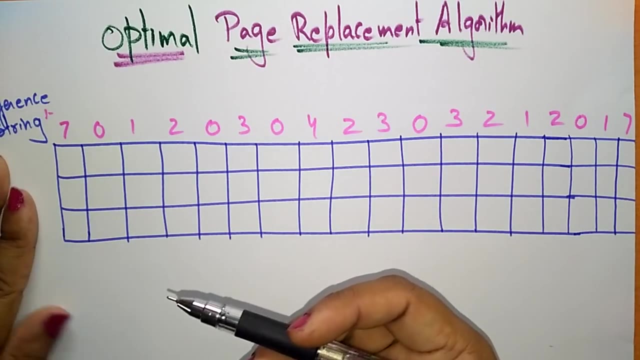 algorithm: or we have to follow the least recently used replacement algorithm, or we have to use the optimal page replacement algorithm. so, based on the user's requirement, you can go for the different page replacements. all got them. so, uh, the hit ratios or the page fault ratios? everything will be based on the reference string taken by the user. 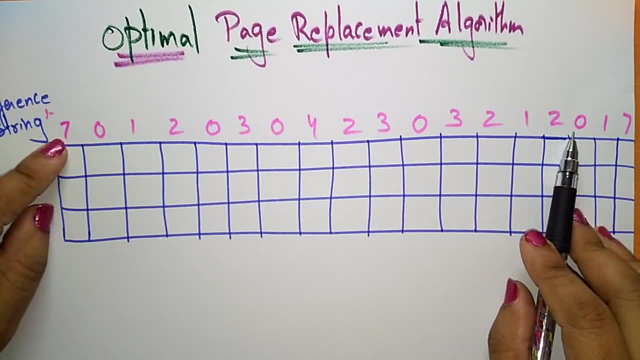 so the user take a string, whatever the string he has taken, and if the those strings or that all uh, the pages that were present in the main memory, then you you will get the less page faults. if those pages are not present in the main memory, then you will get the page faults more, okay, so, 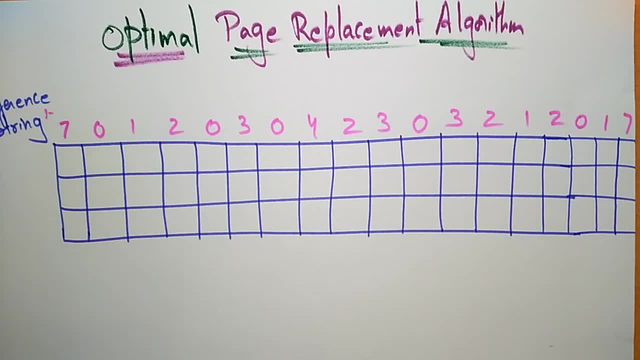 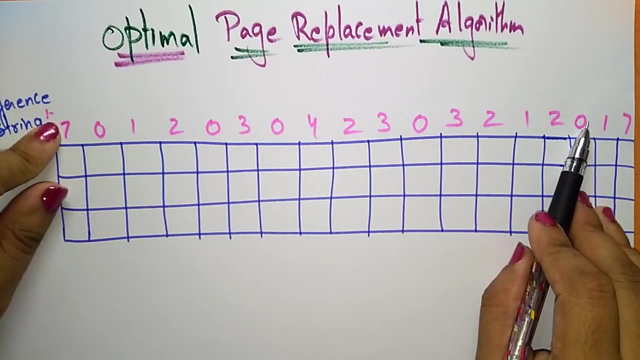 that is the main difference between the different algorithms. now let us see what is the technique that is followed by the optimal page replacement algorithm. so here we have taken the different string. that is a user process. that is the input given. so this is a. the cpu is demanding for these pages in the 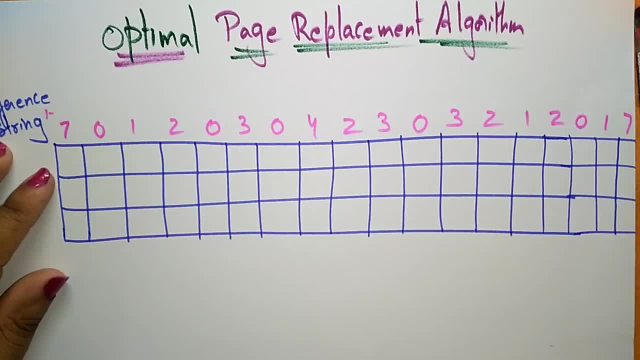 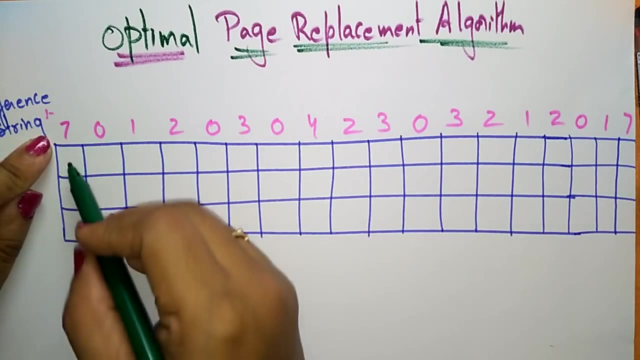 main memory. so now, first it is checking whether this page is present in the main memory. if that page is not present in the ram, then it we call it as a page fault. so first the cpu transmission. the user is demanding for the page 7, so that page 7 is not present in the main memory. 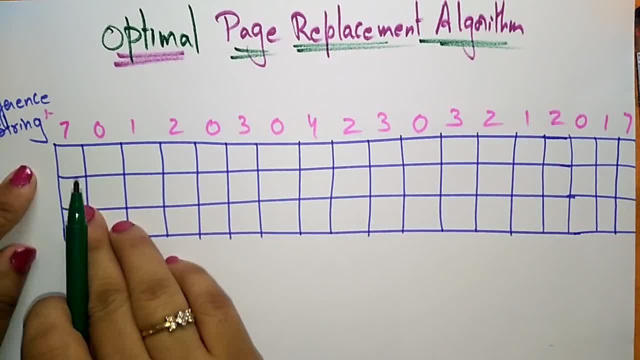 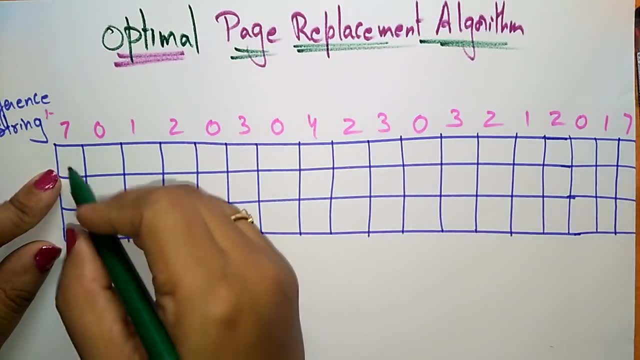 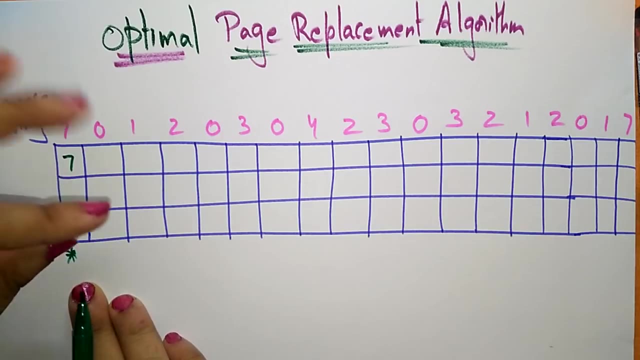 so it's starting. the complete ram is free. so seven is not present so we have to place it for. take it from the disk and uh secondary memory and place it on the main memory. so please, 7. so this comes comes under the page fault because 7 is not present. so we are taking from the. 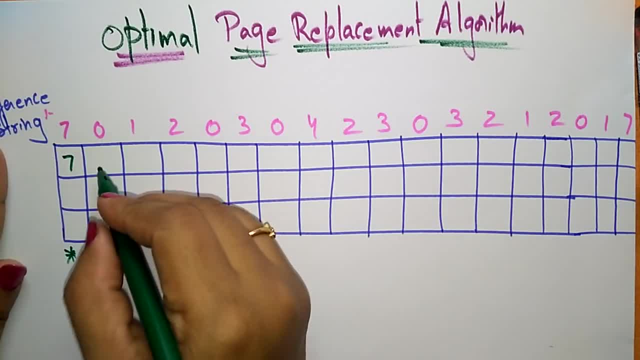 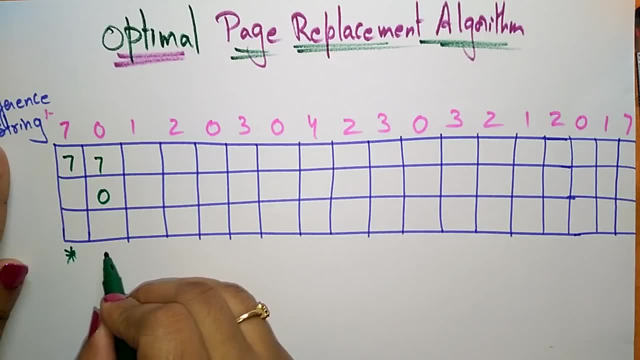 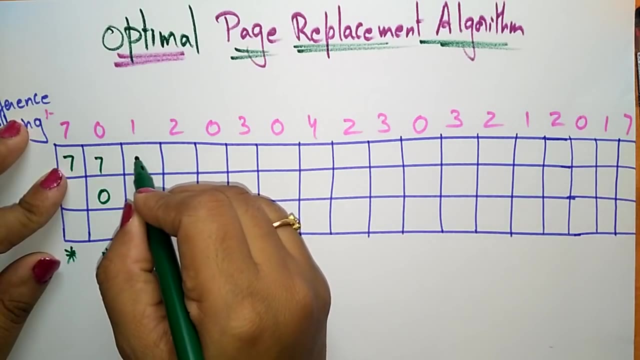 secondary memory and place it in the main memory. so next i have to place 0, 7, 0, so 0 is not present in the RAM. so I have bought that 0 from the secondary memory. now still, the one more frame is free in the main memory. so please, one also. so one is also not present in the 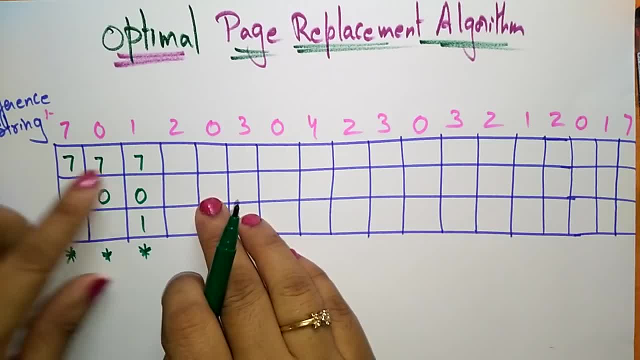 main memory, so we have to board from the secondary memory. now I have to place two, so already the the two is not present in the main memory, so I bought from the secondary memory. but where I have to replace the page, so already the all the frames are full in the RAM, so which page I had to be. 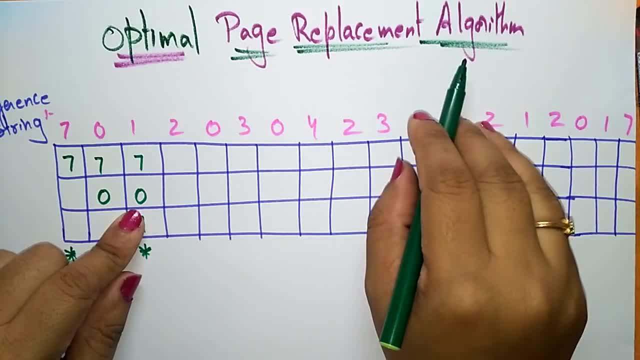 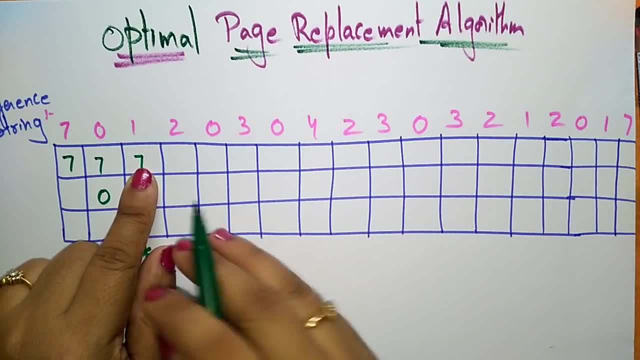 replaced. now, here I have to follow the optimal page replacement algorithm, so the optimal page replacement is saying that. so we have to replace the page which is used later, the later case, later case. so we have to replace the page which is used later, later case. so we have to replace the. 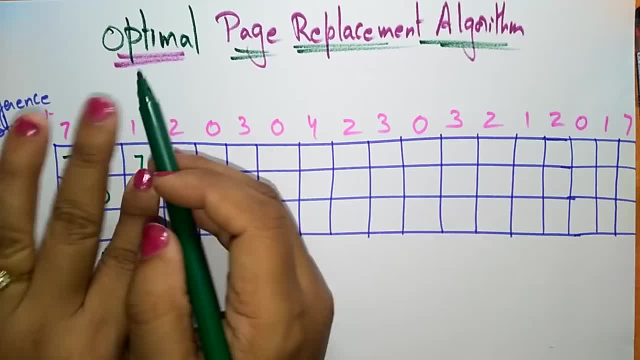 page which is used later- the later case. so we have to replace the page which is used later- the later case. so up to now we have checked. so we have to replace the page which is used later- the later case. so up to now we have checked. so we have to replace the page which is used later- the later case. so up to now we have checked this left-hand side means already used. 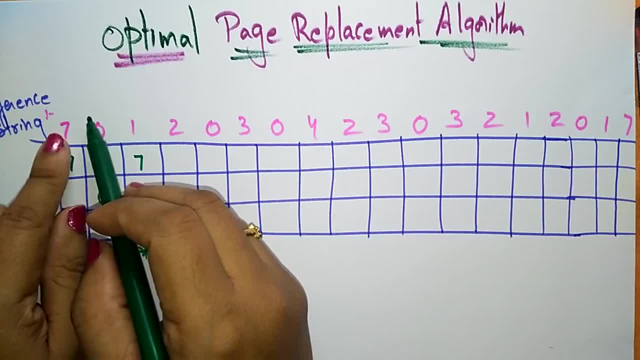 this left-hand side means already used. this left-hand side means already used. pages already refer user reference pages. pages already refer user reference pages. pages already refer user reference pages in the FIFO and LRU, but in optimal page. in the FIFO and LRU, but in optimal page. 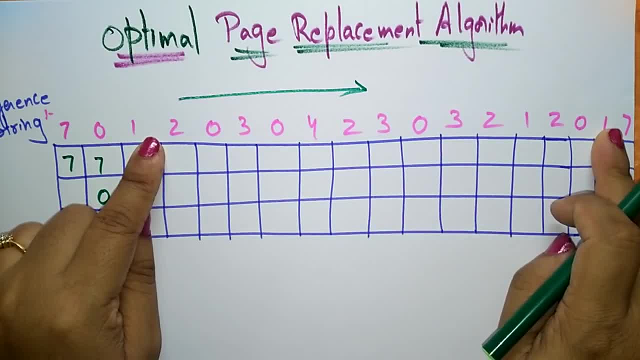 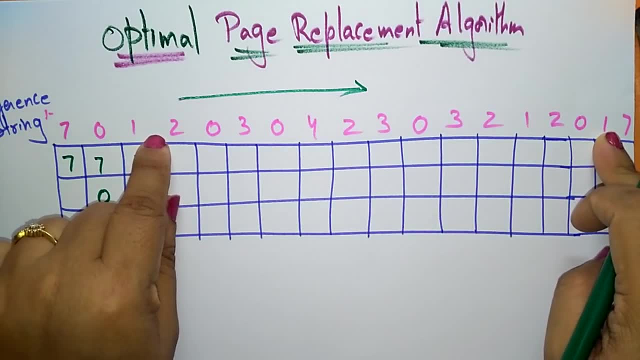 in the FIFO and LRU, but in optimal page replacement. we have to check this site replacement. we have to check this site replacement. we have to check this site means which is not used in longest time, means which is not used in longest time in future. so in longest time in future, we which page reference we are not using, so that page we 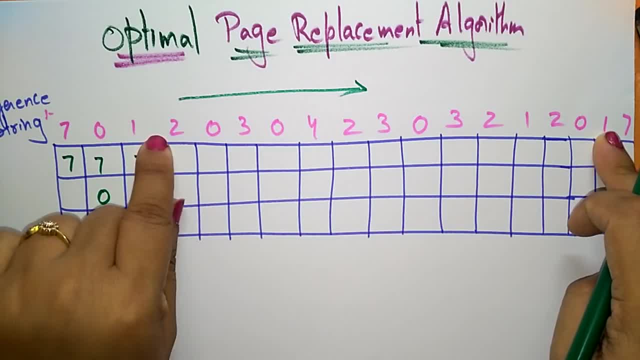 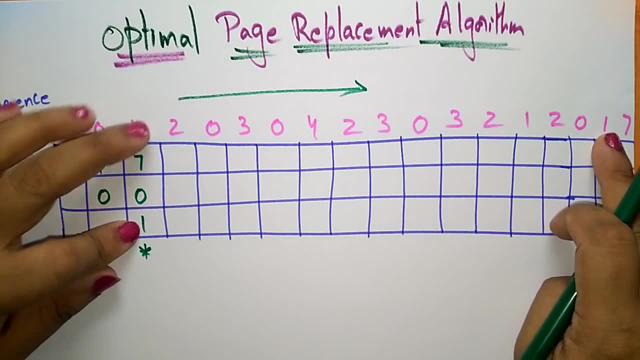 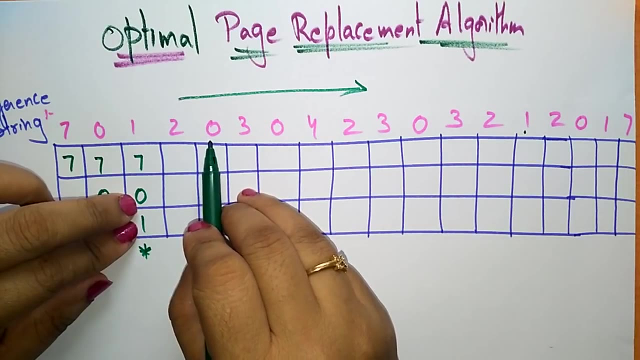 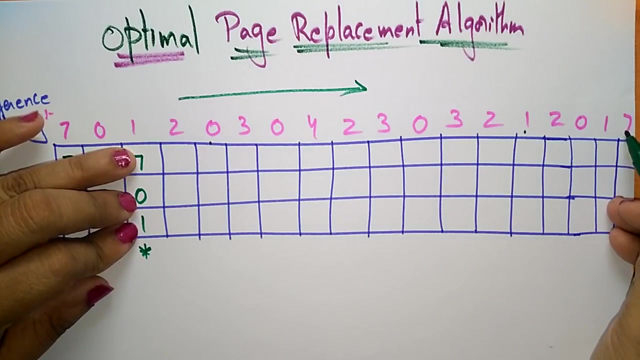 have to be removed. okay, the page that is not used, uh, longer time in the future. so here, if you take one, so one here we are using, okay, and the zero, the zero we are using here. and coming to the seven, the seven we are using at the last. it is the longest time in future, so just replace the seven. 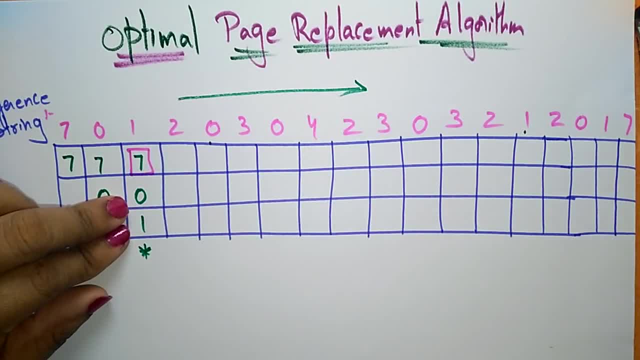 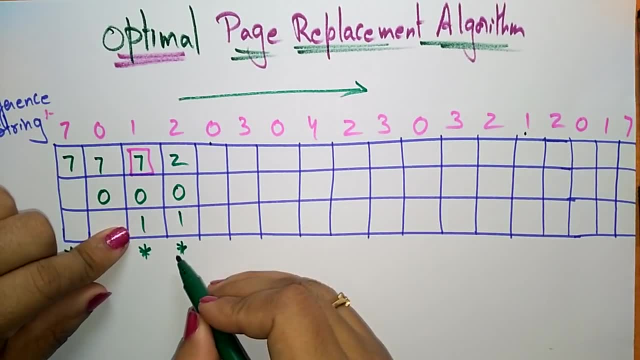 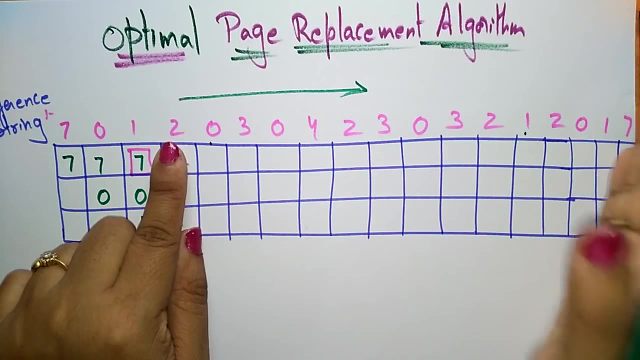 just replace the seven and place two in place of seven. so this is also page fault because two is not present. okay, so the page optimal page replacement is you have to replace the page which is not used. uh, in longest time in future. okay, so the 7 is very longest time in future we are using that 7, so that page we have to be replaced. so 0 means 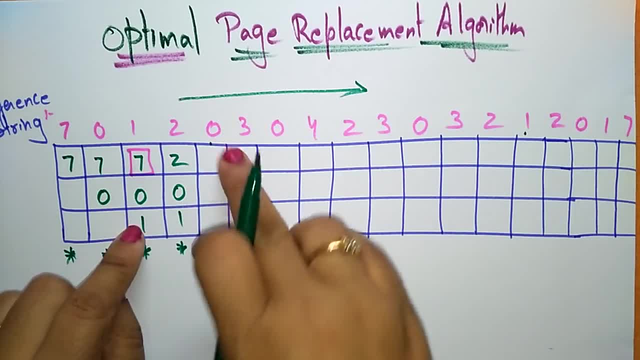 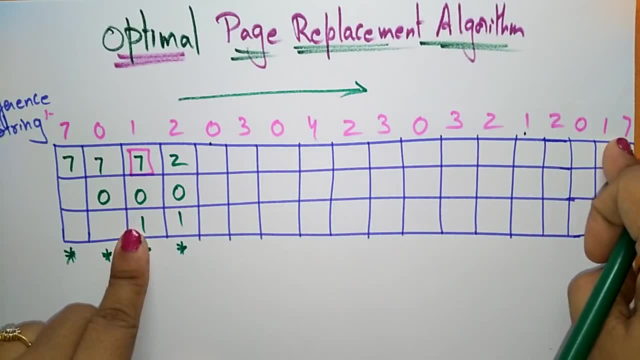 we are using after 2. we are using 0, so don't replace that page. and 1 means when compared to the 7. 1 is using most recently. okay, so the 7 is the longest time we are not using that 7, so just. 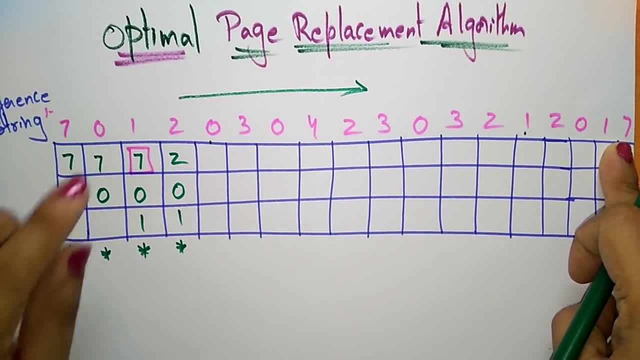 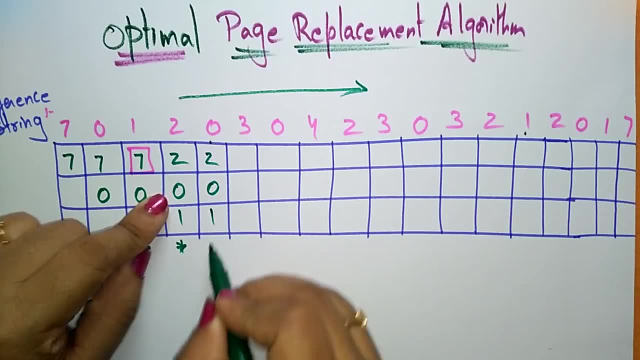 replace the 7. so that is optimal page replacement. now coming to 0. so the demanded page 0 is already present in the main memory, so write as it is. so this is hit. page hit means if the demand at the user's demand page is already present in the RAM. so then you call it as a page hit. now coming to. 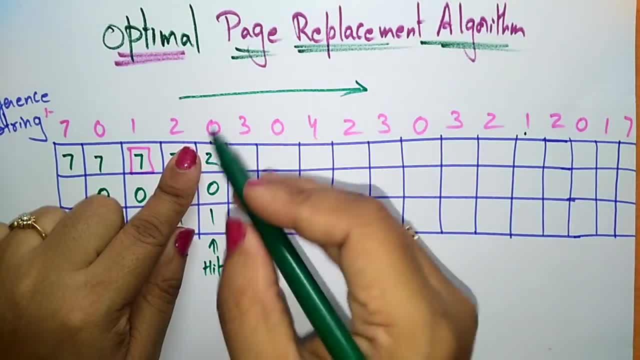 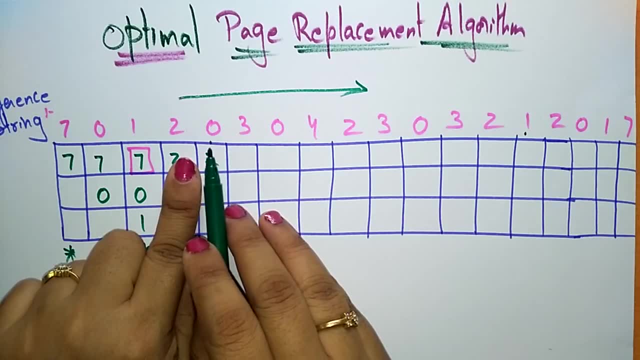 3. so 3 is not present here, so page fault. so we have to bring it from the secondary memory now where we have to place. so now check for the longest time in future which page is used. longest time in future: so 0 is the longest time in future. so 0 is the longest time in future. so 0 is the. 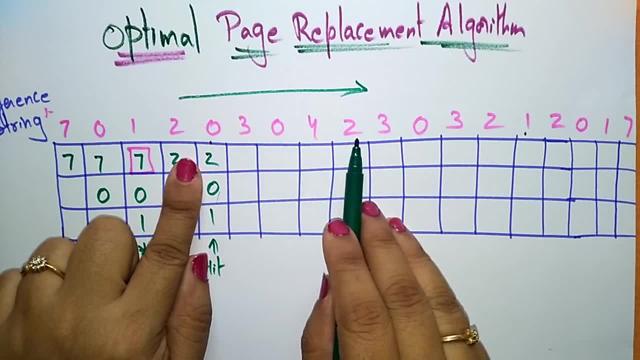 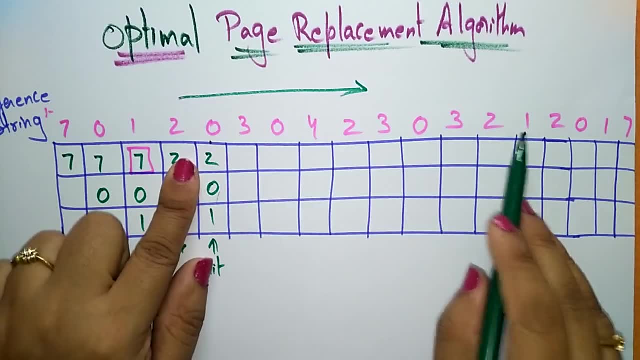 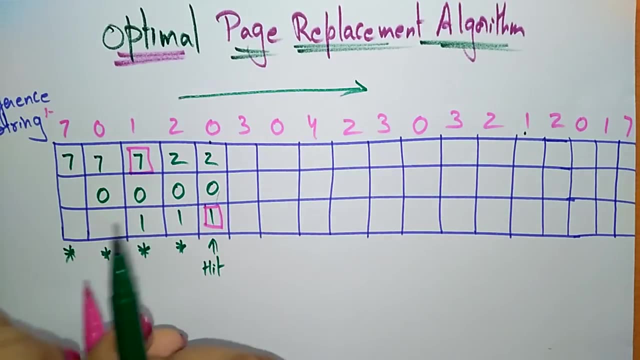 longest time in future. so 2 is using next to the 3, so next 2 is also using next to the 0 and coming to the 1, 1 we are using in the longest time in future, so just replace 1, so in place of 1 we are. 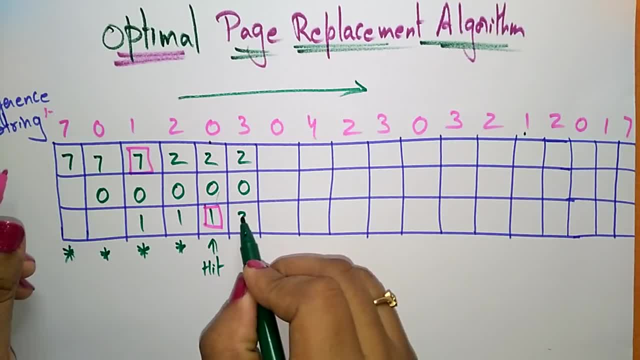 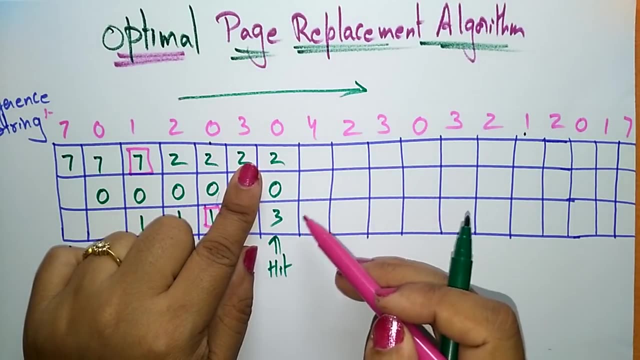 just replacing 2, 0, 3, so 0 is already present in the main frame re, so this is hit. now coming to the 4. okay, so 4 is not eat here, so I have to. this is a page fault so I had to brought from the. 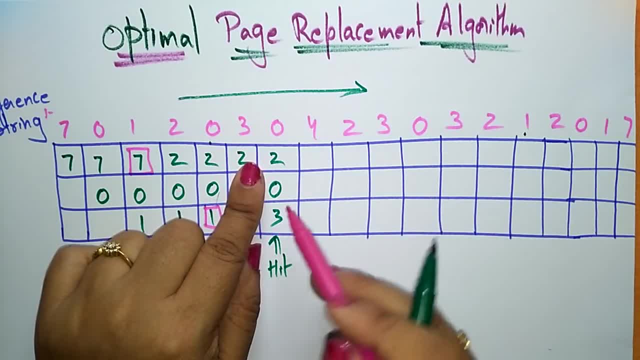 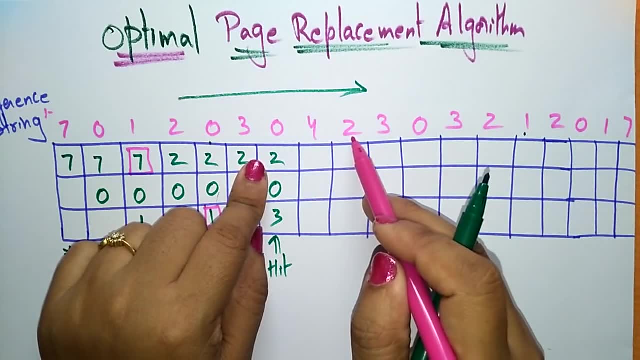 secondary memory now which page I have to be to place the 4. so now checked in the longest time in the future. we are using the 2 E's next to the 4, we are using 2, so don't replace to next three is also I'm using next to the 2, so the 0, the zero E's when compacted, 2 and 3, 0 E's also. 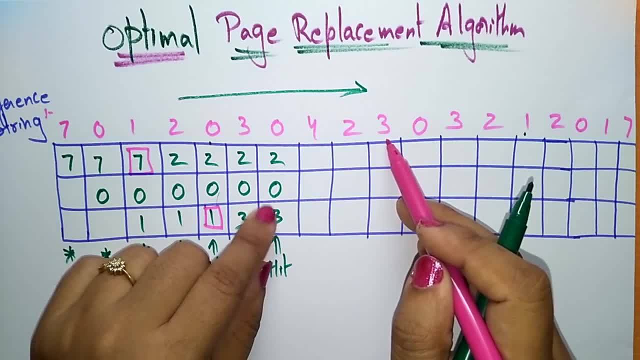 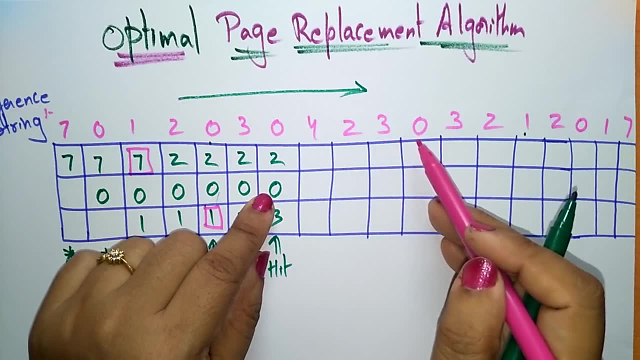 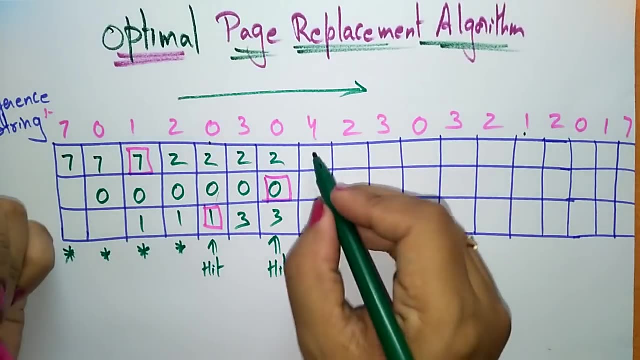 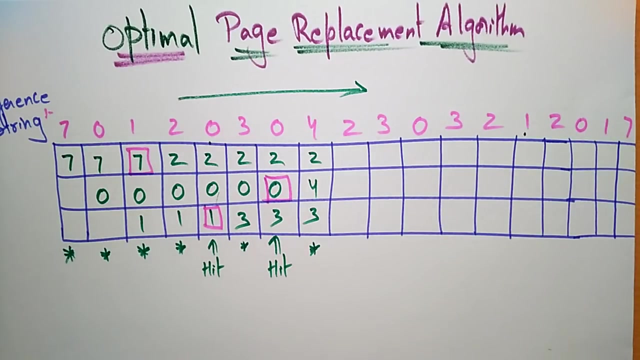 are using next to the 2, so the 0, the 0 E's when compacted, 2 and 3. 0 is the length of the page, you the longest time in future. we are using that reference string, so just replace the 0. so in place of 0 I had to write 3. so this is also page fault. ok, now 2. 2 is 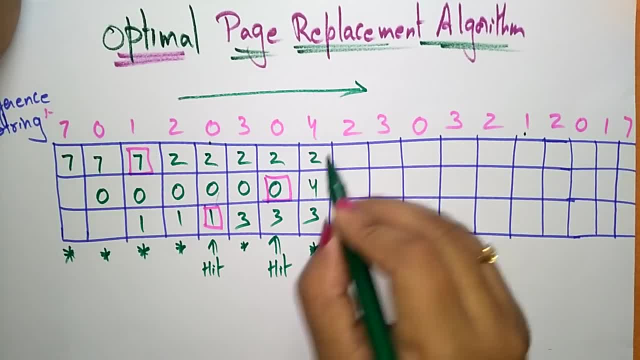 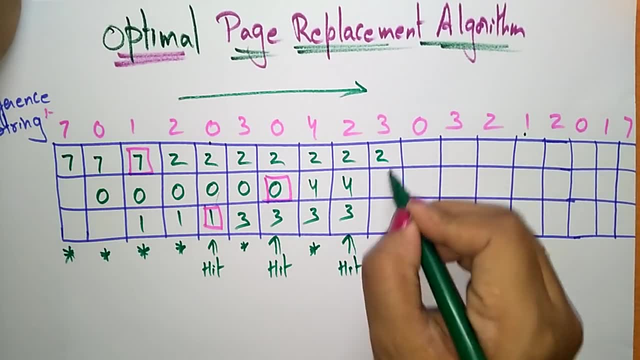 already present in the main memory. the demanded page is already present in the main memory, so just simply write that and mark it as a hit. now coming to 3: 3 is also present in the main memory. that is around. so hit now place 0. so 0 is not. 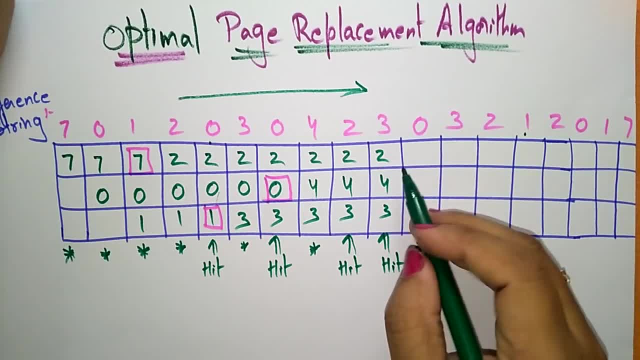 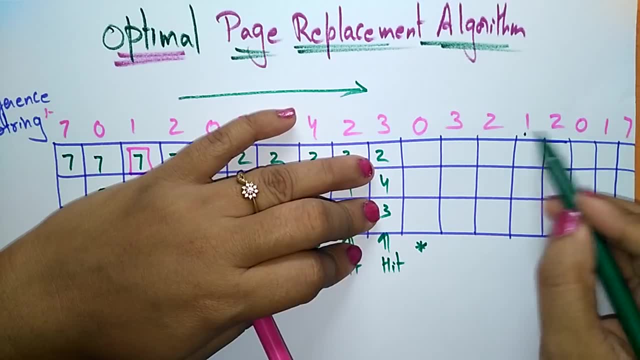 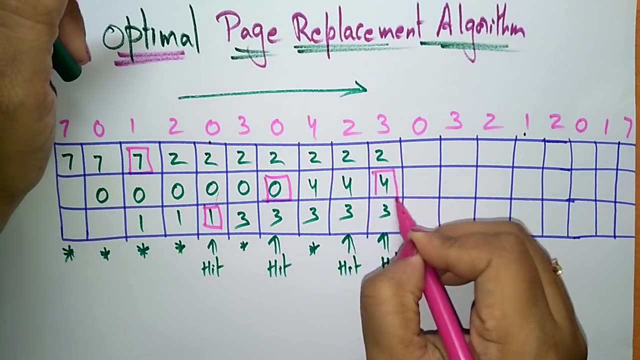 present here. so page fault. so page fault. so which page I had to be replaced from 0? the 3 is next used, 2 is next used, so 4 is not here. so if there is not, the 4 is not present here, so just replace that because it is not using so longer. so in. 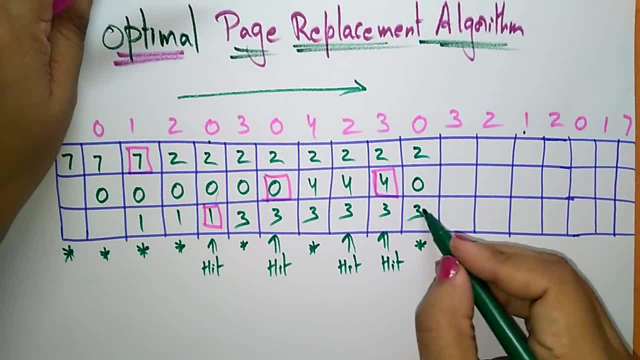 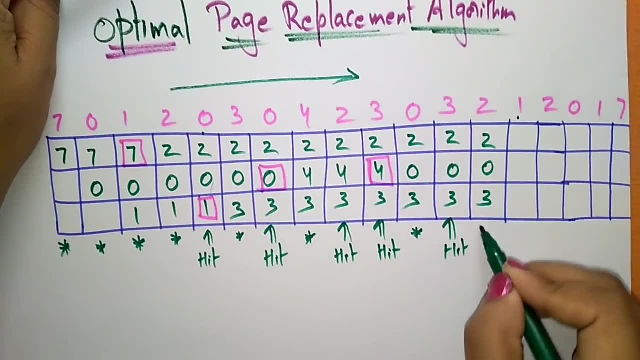 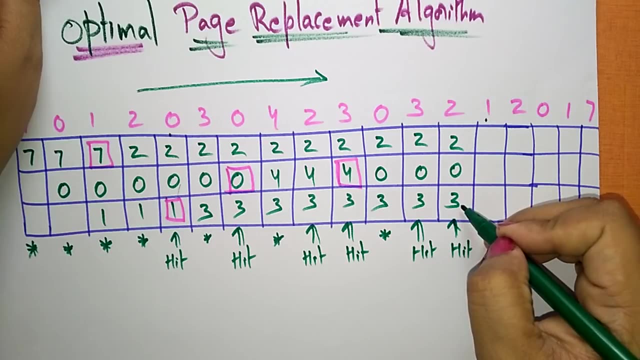 place of 4 just write 0, 2, 0, 3. so 3 is already present. hit 2 is already present in the main memory, so this is also hit next coming to 1,. 1 is not present in the main memory, so I had to. 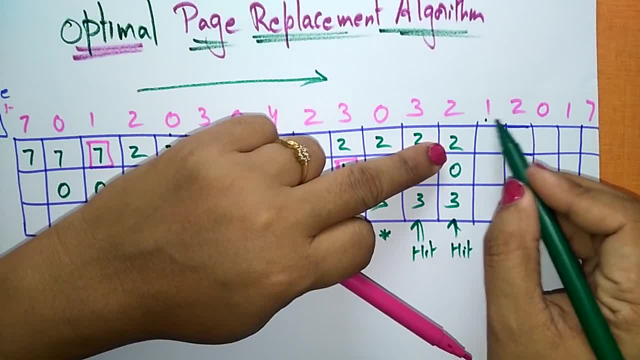 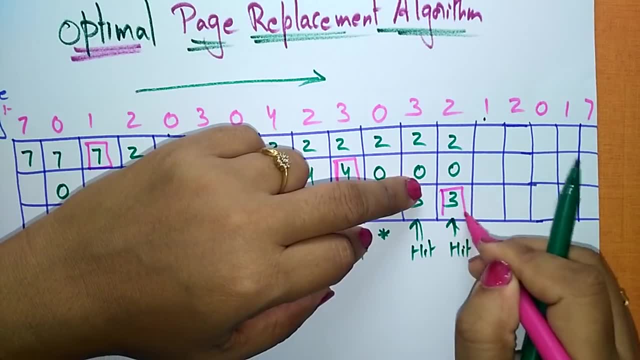 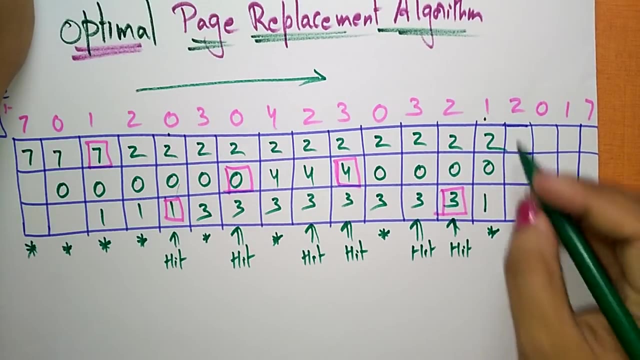 replace the page. which page I had to replace. so 1 after I am using 2. ok, next is 0, so 3 is not here, so just replace the 3 in place of 3. I am writing 1, 0, 2, page 4, so 2 is already present in the main memory. so 2, 0, 1. this is hit and 0. 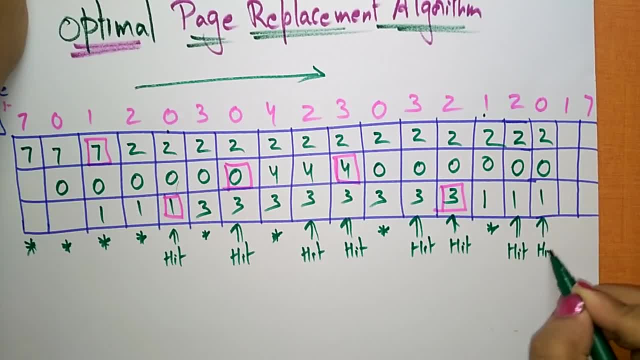 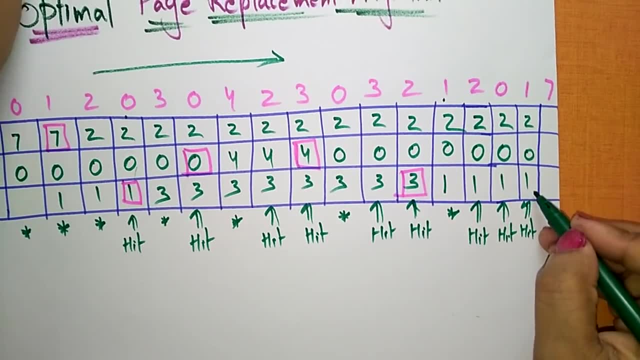 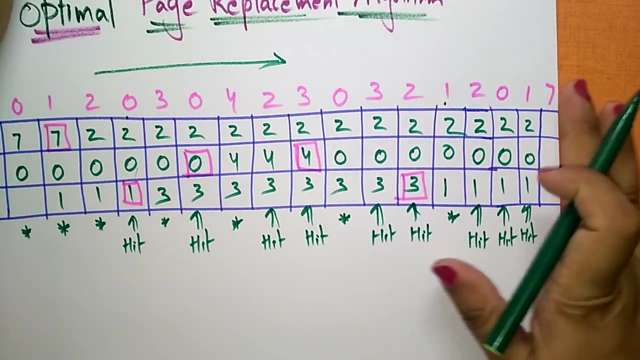 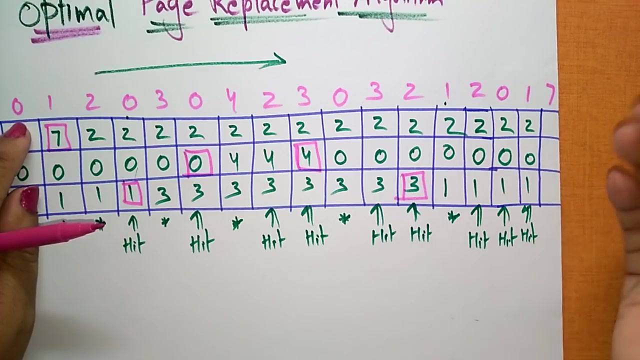 is already present: 0, 1 hit. 1 is already present. so 2 0, 1, simply write. as it is now coming to the 7, so which page I had to be replaced? okay, so like this here. it is going like this here. next. the strings coming to next is 1, or else you just. 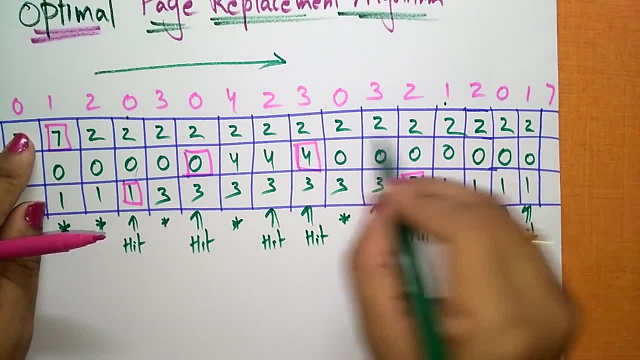 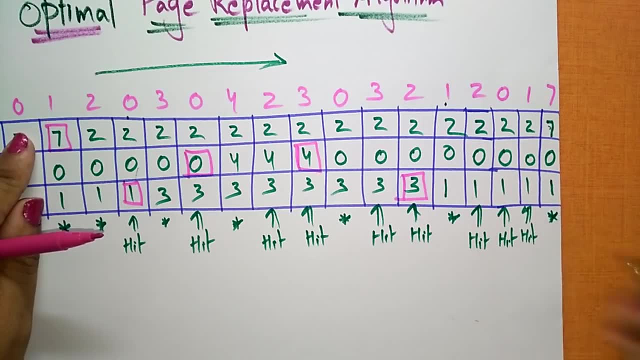 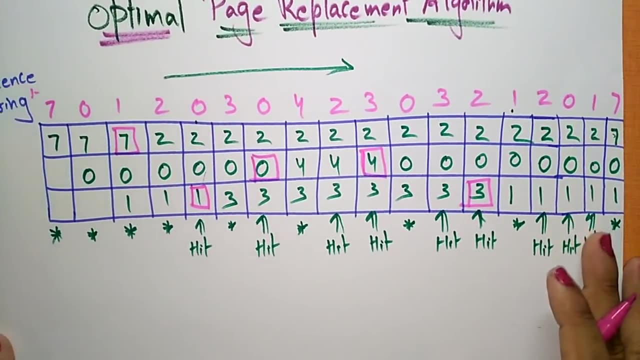 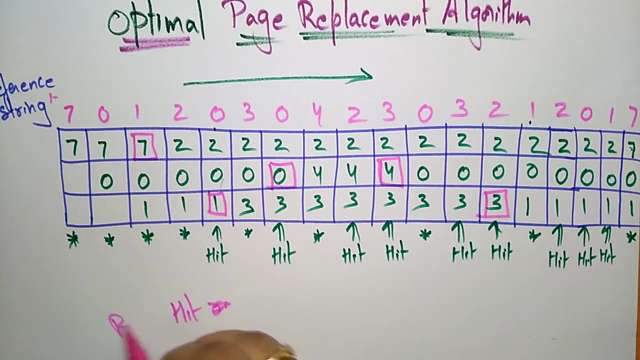 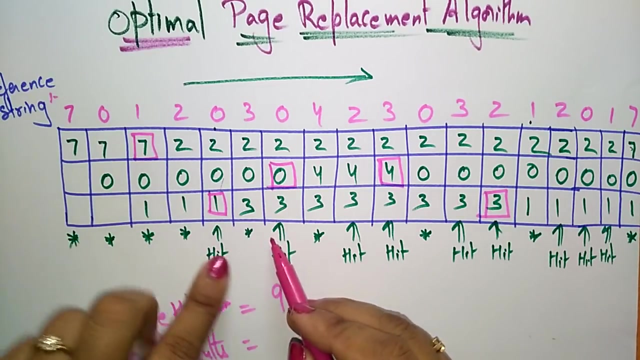 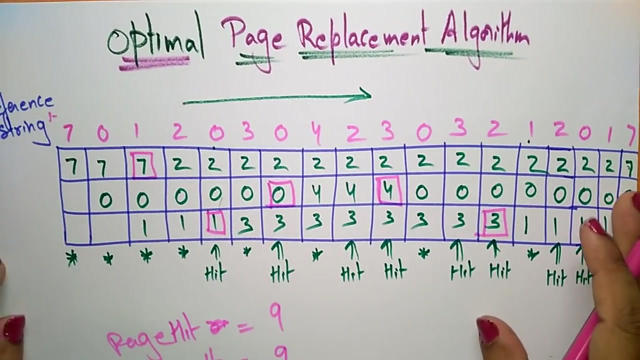 simply replace the item which we are using so longer time. that is the 7, 0, 1. so this is page fault. okay, so this is the optimal page replacement algorithm. so here then, what is the number of hit ratio? So let's page hit. So the page hits are 1, 2, 3, 4, 5,, 6,, 7,, 8, 9.. 9 page hits: What are the page falls: 1, 2,, 3,, 4,, 5,, 6,, 7,, 8,, 9.. So 9 page hits and 9 page falls in this reference string. 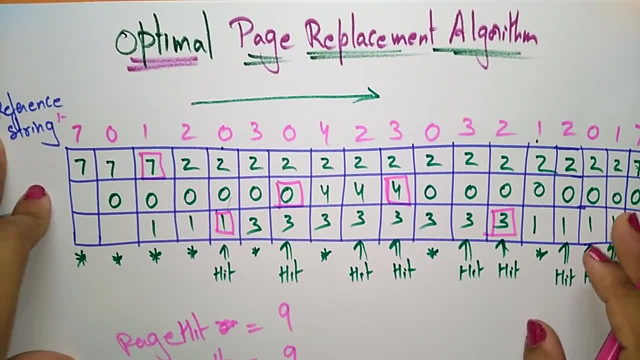 So the hits and falls will be changed based on the reference strings that the user is given. So this is about the optimal page replacement algorithm. Thank you.